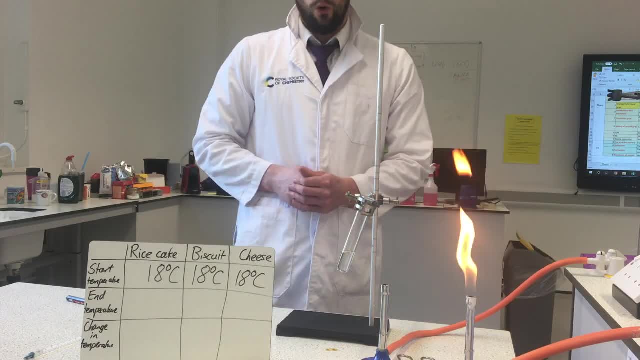 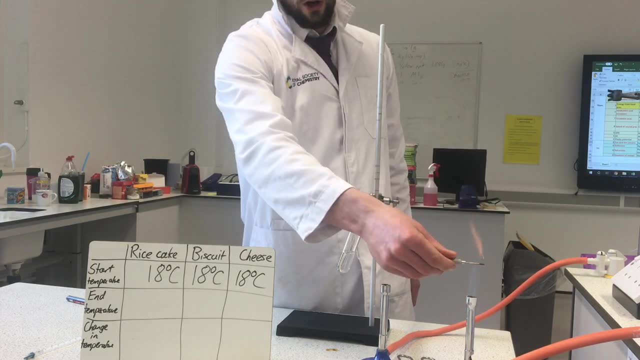 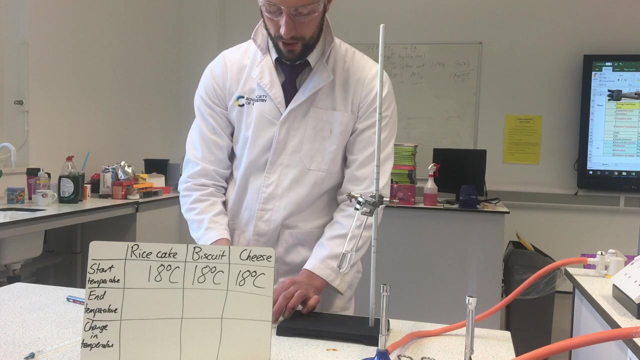 I've written down the start temperature as 18 degrees for all three of my experiments. What I'm going to do here is I'm going to take a pin, I'm going to get it nice and hot to help it stick into my food, and then I'm going to put my food on the pin, and the first food I'm using is rice cake, as I'm sure you can see in my table. 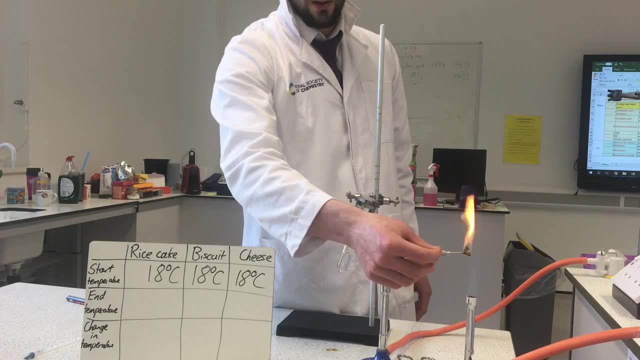 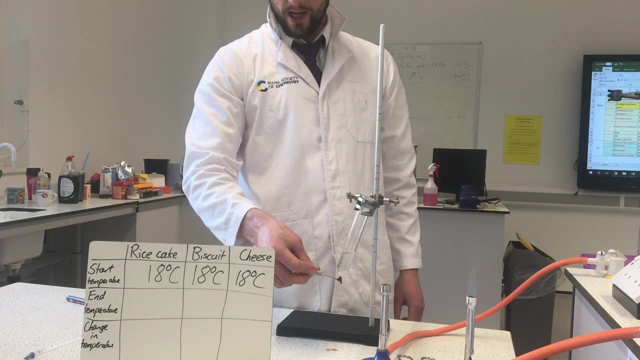 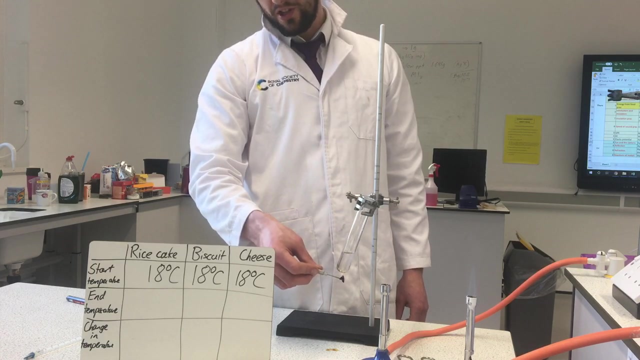 I light the rice cake on fire and then, once it's burning, I'm going to use it to heat the water. Now the burning is transferring the chemical energy in the rice cake to thermal energy, which is heating the water. When I measure the temperature of the water, I can see how much thermal energy has gone into it. 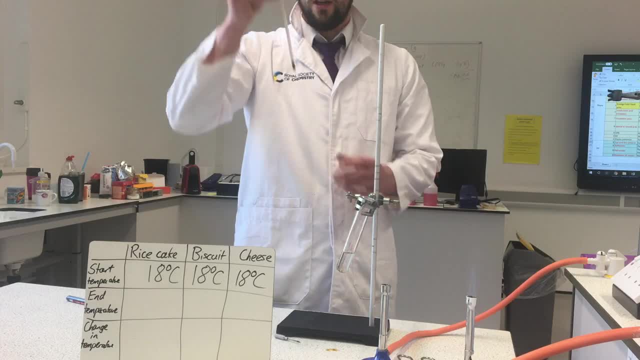 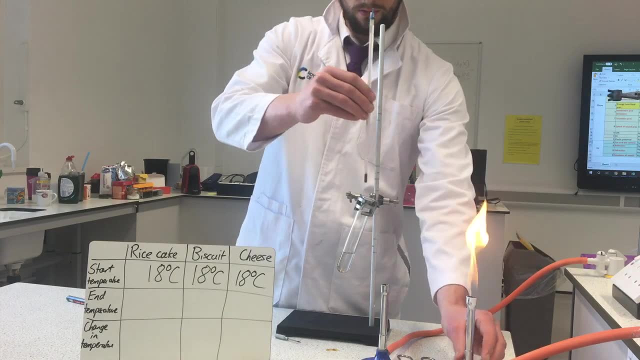 That burned up very quickly. I'm now going to take my thermometer and see what the temperature of the water is. Remember it started at 18 degrees. It is now- Oh, that's definitely gone up. I can see the temperature shooting up nice and quickly. 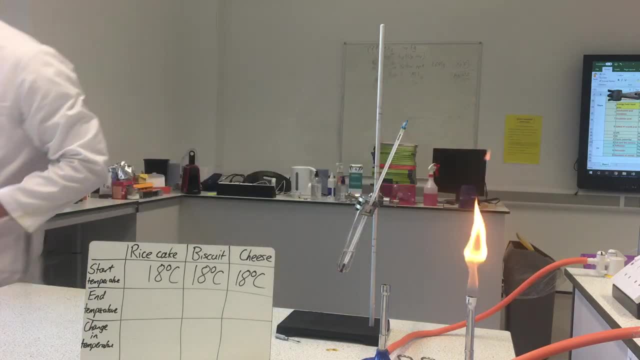 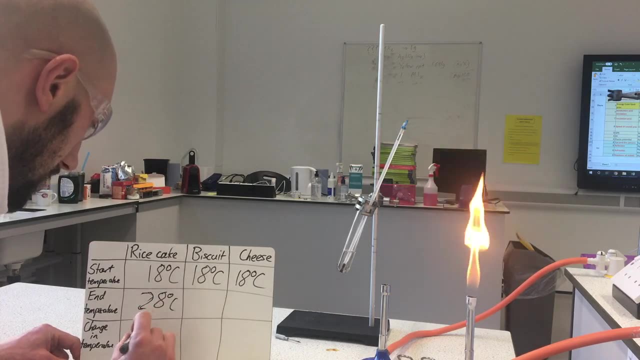 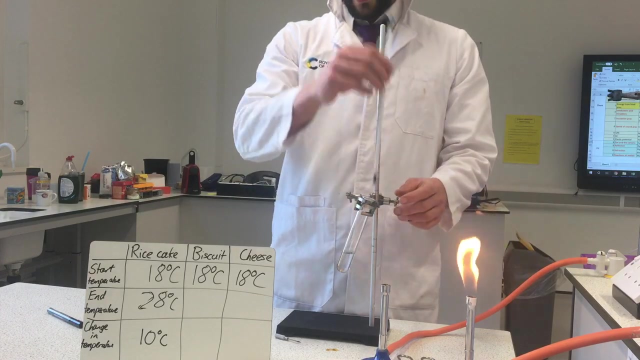 It's now gone up to 28 degrees. That's a change of 10 degrees. 28 degrees, That's a change of 10 degrees. So there was enough chemical energy in the rice cake to heat up the water by 10 degrees. 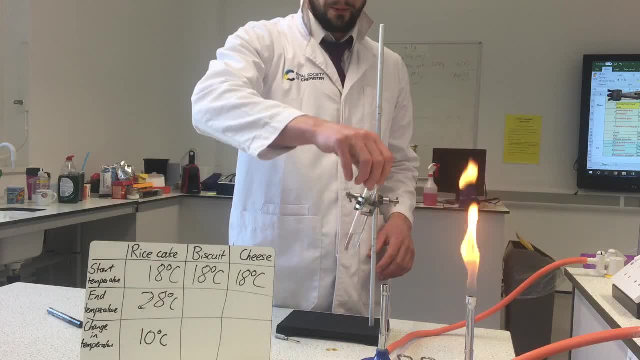 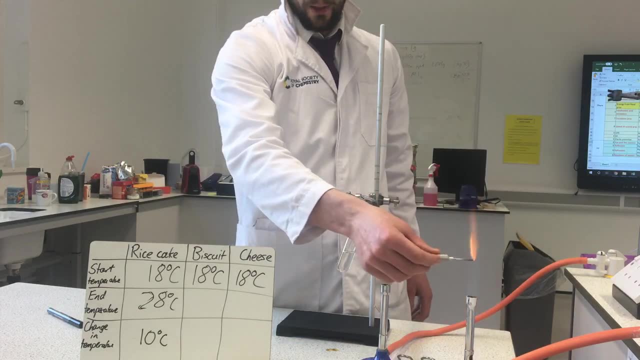 I'm going to put a fresh set of water in, and I'm going to do the same with a different food this time, So I'll take another pin. I'm going to heat it in my hot Bunsen burner flame, Stick it into- this time a piece of rice cake. 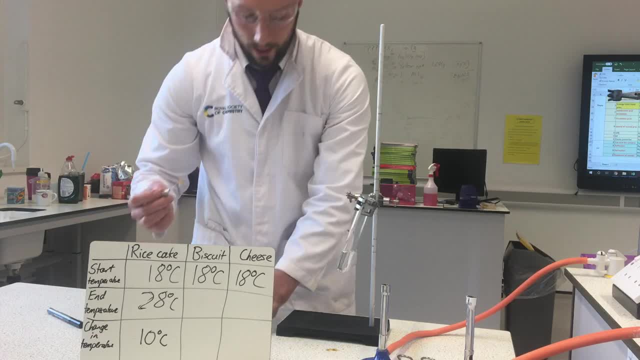 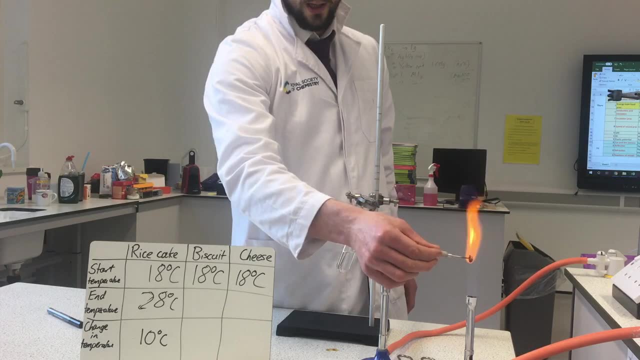 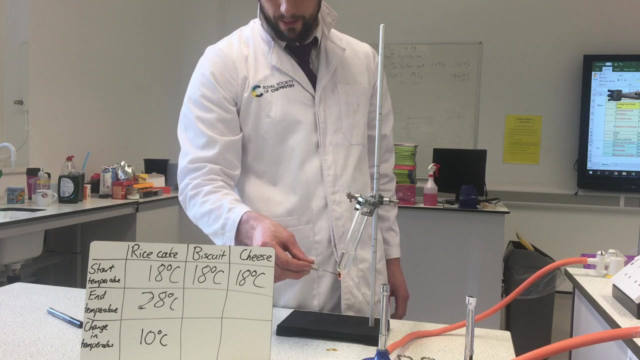 This time a piece of biscuit. Now, the rice cake contains lots and lots of carbohydrate. We know that rice has the nutrient carbohydrate in it. The biscuit also contains some carbohydrate, But as well as carbohydrate, the biscuit contains some sugar and some fat. 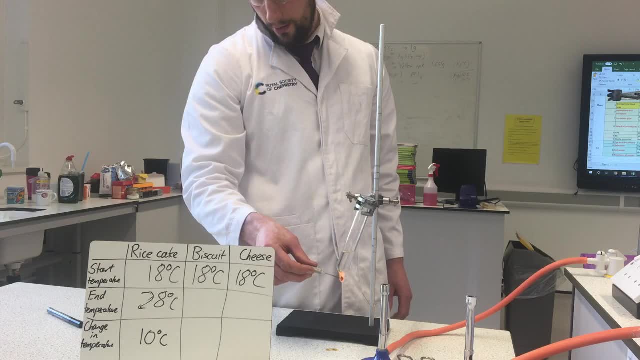 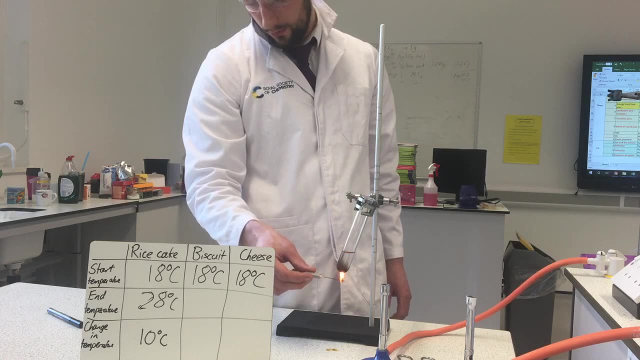 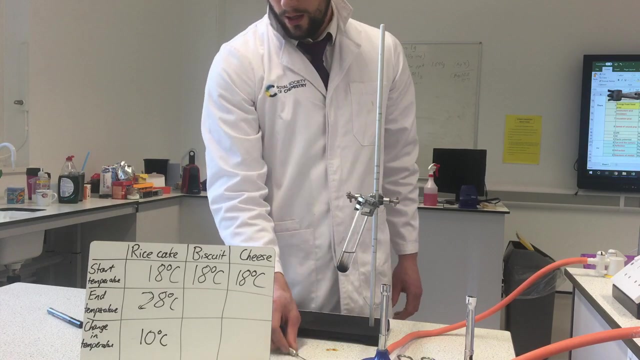 So it's got slightly different nutrients in it. We'll see how that affects the amount of chemical energy it's got in it. Wow, that biscuit is burning really well And that's about all. So that's the chemical energy from the biscuit. 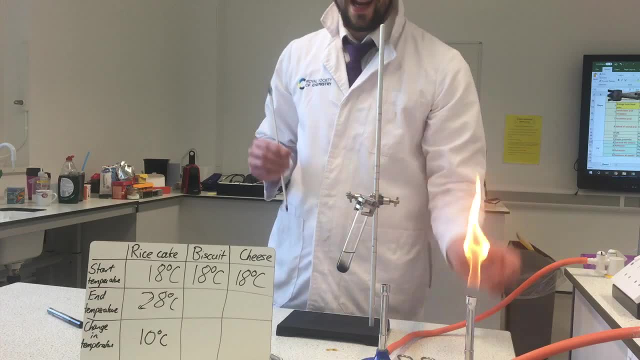 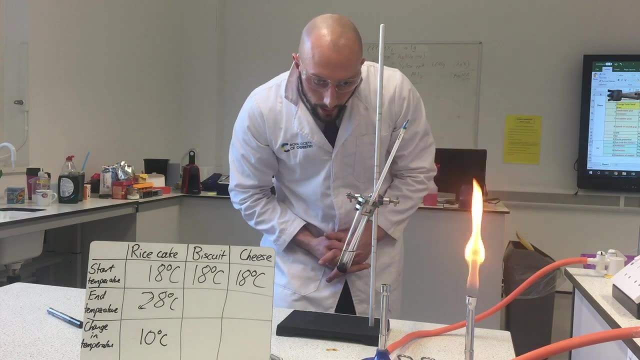 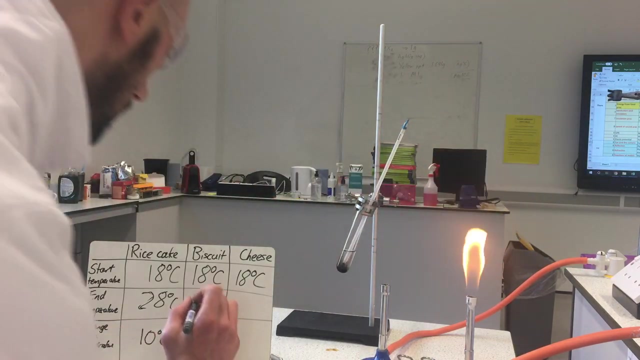 Has been transferred into thermal energy in the water. That's a heating transfer. The water has warmed up. Yep, the temperature is rising quickly. It's gone to 33 degrees. it's gone up to- Oh, look at that, That's very neat. 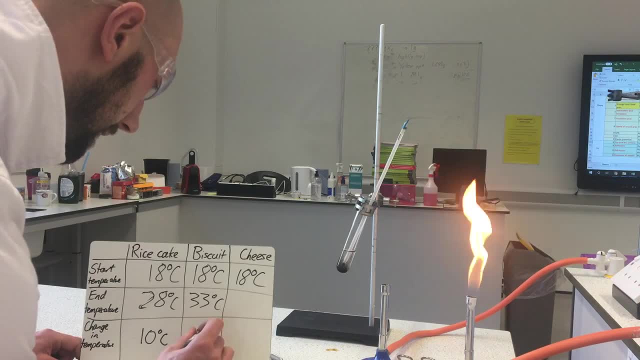 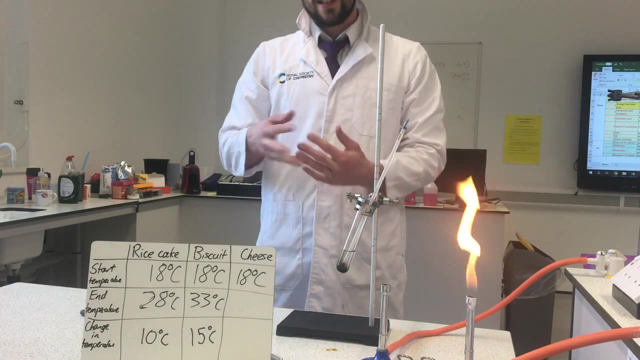 So far at the moment I've got 10 degrees and 15 degrees for my change, So there's a bigger change in temperature from the biscuit. So that told me that the biscuit had more thermal energy than the rice cake And I'm using the same mass of all of the foods. 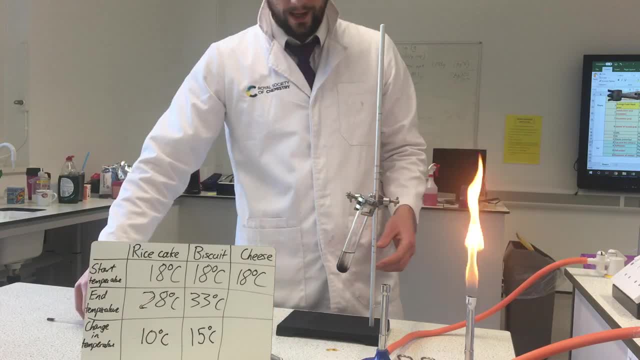 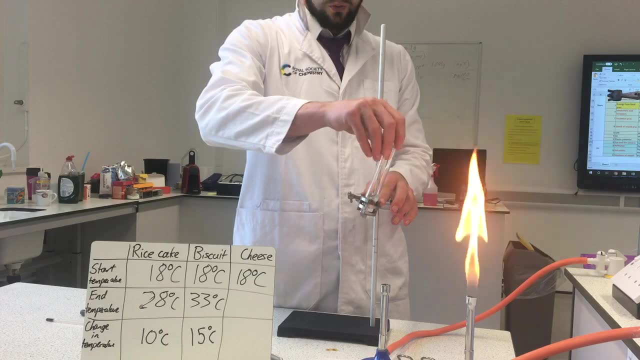 Even though the pieces are different sizes, I weighed them carefully. That's a control variable. Let's do my last one. I've got my last thing of water. It's 20 mils of water at 18 degrees. More control variables. 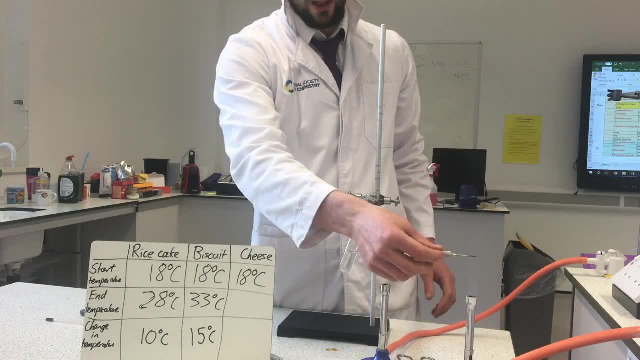 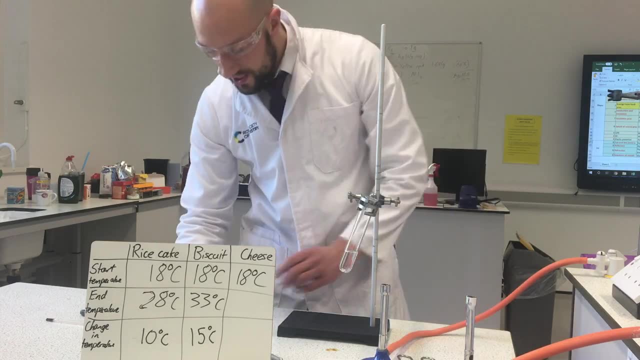 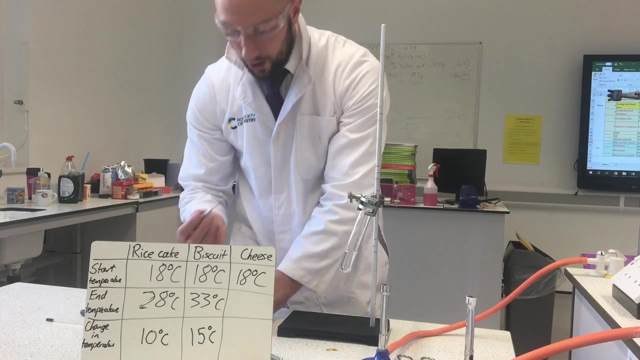 I'm going to take my last pin, Heat it hot So I can stick it into my food. Now my pin is nice and hot. I'm going to stick it into my last food, Which is a piece of cheese. Now, cheese contains a little bit of carbohydrate and a little bit of sugar. 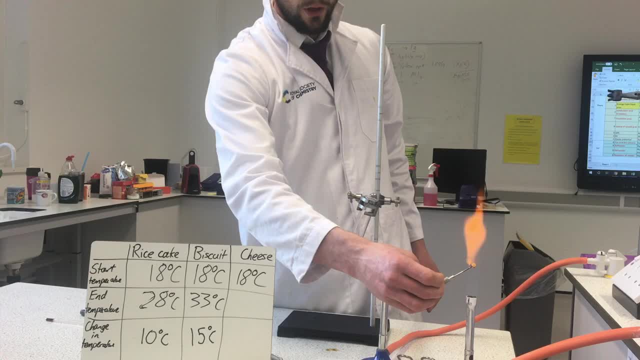 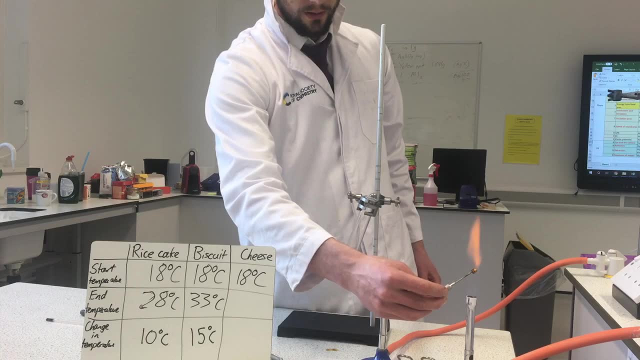 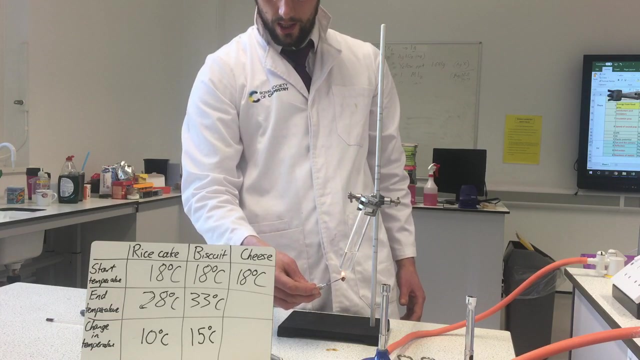 But it's pretty much all fat. It's a different nutrient to what we had in the other ones, So let's get that cheese burning. Yep, my cheese is burning nicely there. I'm going to use the cheese to heat the water. 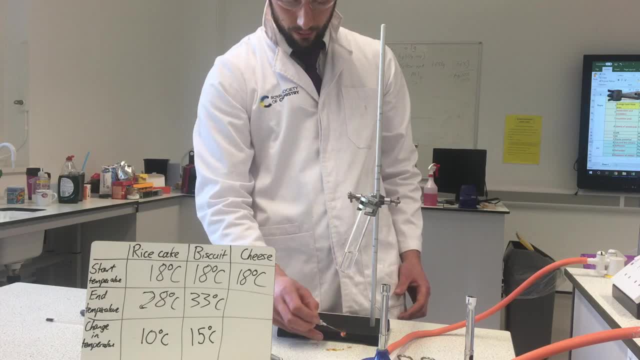 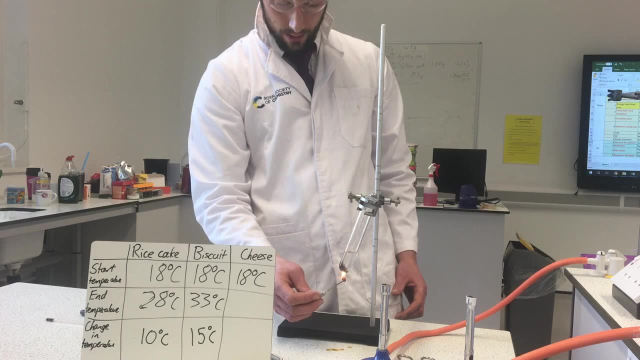 Oh, it's fallen off the pin. That happened earlier as well. Let's see if I can keep it going. There we go. It shouldn't be too bad. So remember, the cheese has got lots and lots of fat in it. The biscuit had fat and sugar and carbohydrate. 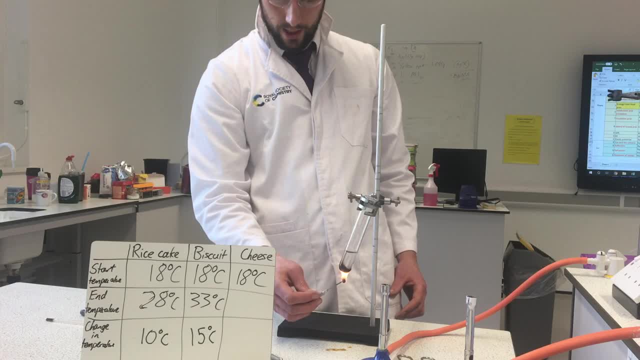 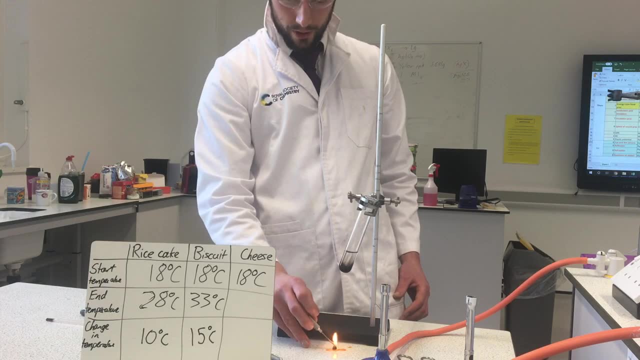 The rice cake had basically just carbohydrates in it. We've got the same mass of all of the foods. We've got the same volume and temperature of the water. every time It keeps falling off, doesn't it? It's because the cheese is melting. 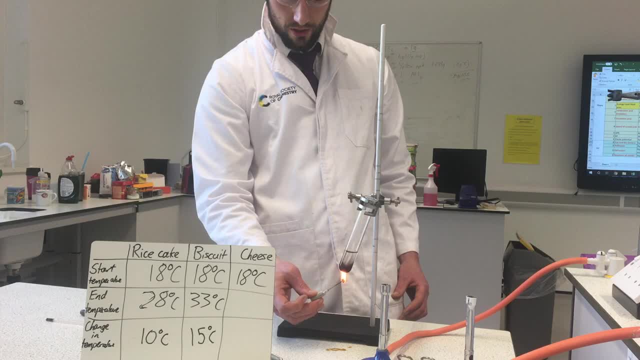 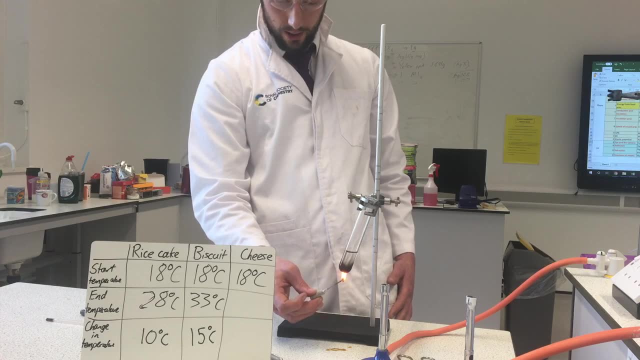 We all know that if you put cheese under the grill, you get nice melted cheese on toast. Well, that's what's happening when I'm burning it here, And that looks like it's nearly finished burning the cheese. It's going for a long time, so I think it's transferring a lot more energy than the others.